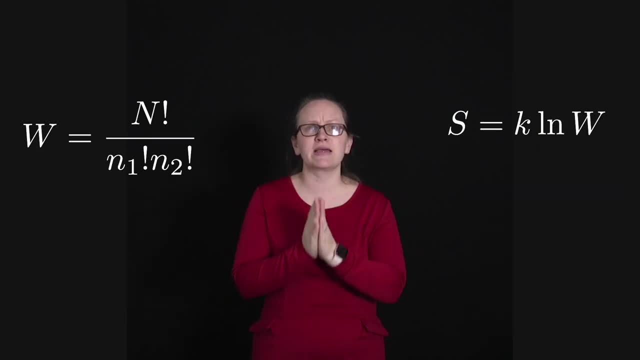 We'll see an example in just a minute. Okay, but it does make sense that we've got a logarithm in there, because if you think of two individual systems and combining them, when we combine them, you can see that we have two logarithms. When we combine them, you can see that we have two. 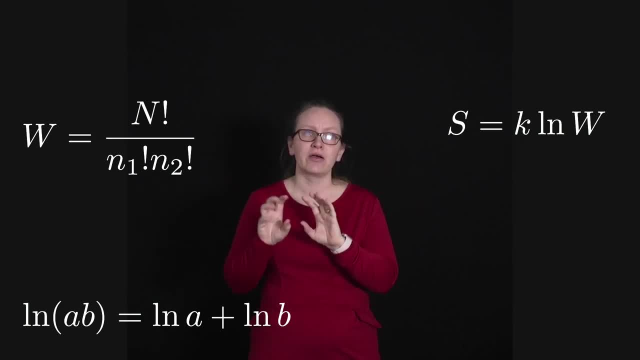 logarithms. When we combine them, you can see that we have two logarithms. When we combine them, the entropies of those two systems add together, while the probability of specific states is calculated by multiplying the individual probabilities together, and logarithmic functions have this property. We know that log of a times b is equal to log of a plus log of b. 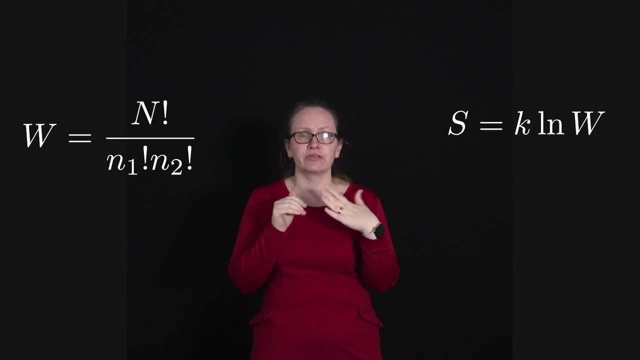 Now, one thing that you should be aware of is because factorials can get really big really quickly. sometimes your calculator can't cope with it and will have an overflow. In that case, it's useful to make use of an equation that Stirling came up with. If you've heard of Stirling engines before, it's not the same Stirling. this is a. 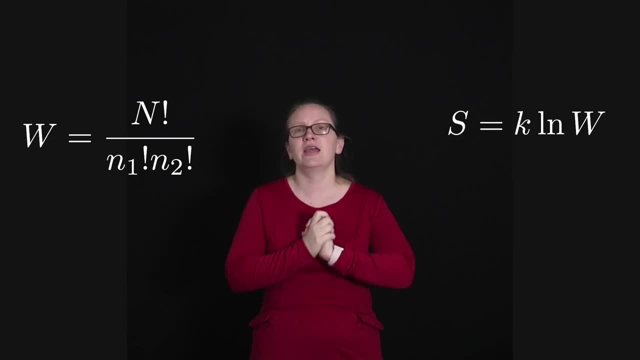 different Stirling Stirling, who was a mathematician. he showed that log of n factorial is equal to n log n minus n. Okay, so that's written so that you can see it clearly. So let's see an example of how we calculate the entropy now. 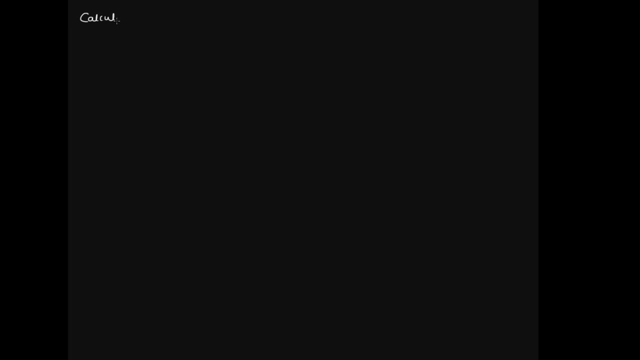 Okay. so what we're going to do now is calculate delta s in two ways. for isothermal free expansion, where the gas doubles its volume, Okay, so this first way, just the. using the heat transfer, we showed that the change in entropy was equal to s of the final state minus s of the initial state, which we showed was equal to nr. 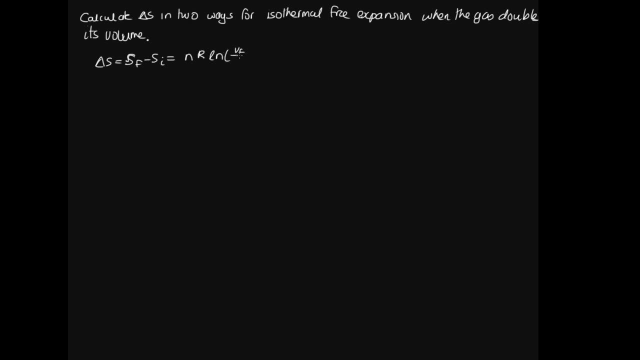 times log b final over v initial plus n cv times. log of t final over t initial. And because this is an isothermal free expansion, the temperature's not changing, So this is log of one. so this whole term here is equal to zero and the final volume is double the initial volume. so this is equal to nr. 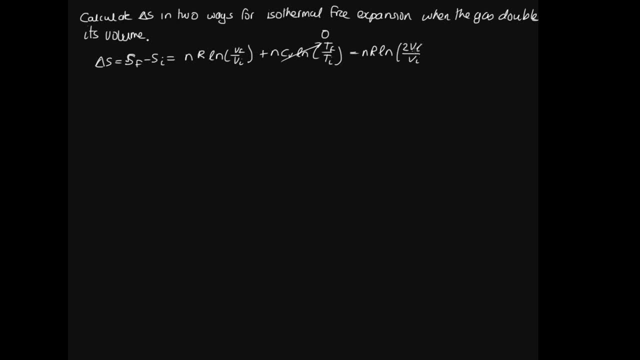 log 2: v initial over v initial. these cancel out and we have nr log 2.. Okay, so we've calculated it in our way, where we're considering heat flow and temperature. Now we're going to calculate it by counting the number of states and using Boltzmann. so, using Boltzmann. 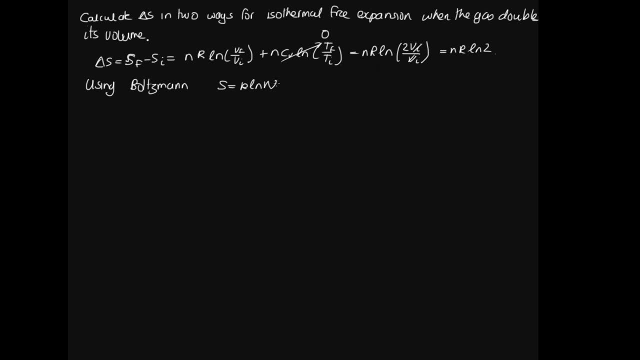 we know that s is equal to k log w, where w is the multiplicity of states. so initially, if we've got some total volume, we've got n particles on the left hand side and none on the right hand side. this is initially, and then afterwards the particles have evenly distributed themselves. 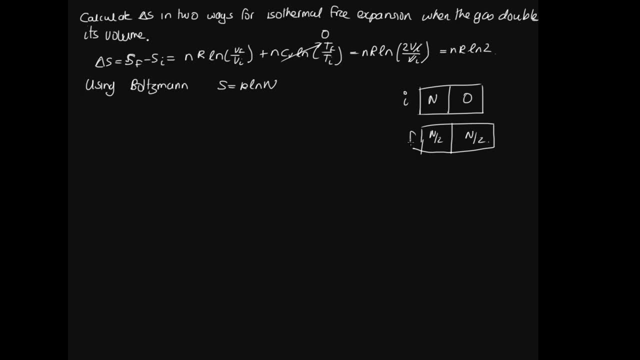 between the two sides. so we've got n on two here and then onto here, and this is the final state here. so now we work out the change in entropy between these two states here. okay, so to do that we we need to know w for these two states, so w for the initial state. well, just remember that w. 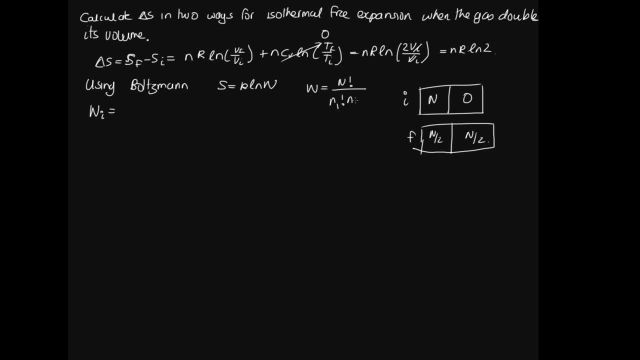 is equal to m factorial. and then for the initial state we'll just remember that w is equal to m over n1 factorial, n2 factorial. in this case we've got n factorial over now n1- there's capital n in there, so that's n factorial and there's none in here, so zero factorial, so that's n factorial. 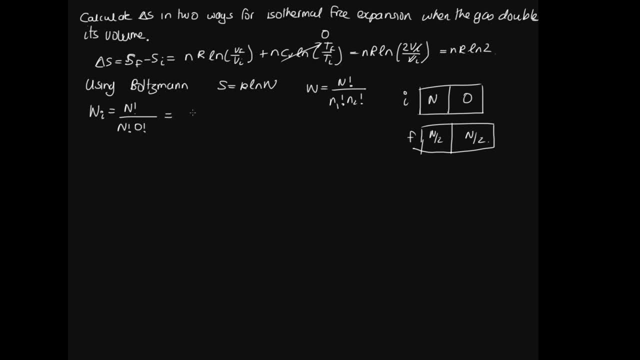 divided by n, factorial divided by one, and so these cancel and we get one as the initial configuration of states, so we can actually calculate the initial entropy. it's equal to k log of one. log of one is zero, so it's actually zero, so the initial entropy is zero, okay. the 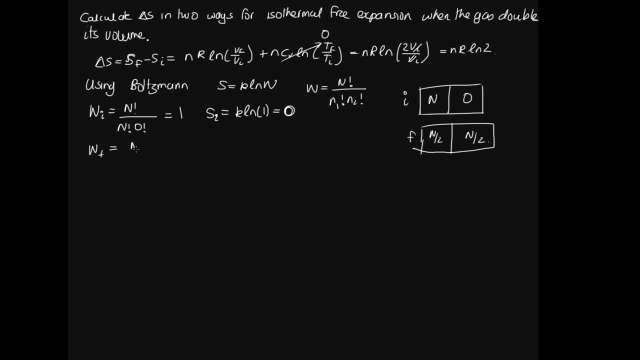 multiplicity of states. for the final state we've got n factorial over n onto factorial times n onto factorial. so substituting this in the final entropy is going to be k log of n factorial over n onto factorial- n onto factorial. okay, now this is a log, so we can use our log. 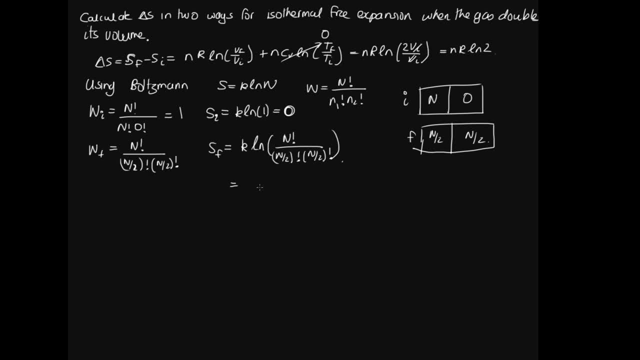 rules: when we divide by logs we subtract the logs. so this is k log n factorial minus k log n onto factorial and this thing's all squared. and hopefully you remember that when you have a square inside the log you can pull the two out the front. so this is equal to k log n factorial. 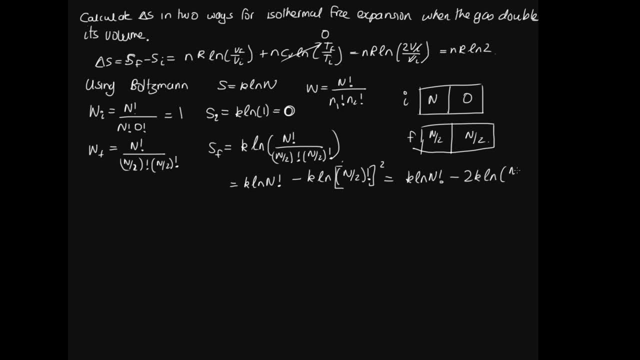 minus 2k. log n onto factorial: okay. now, in order to simplify this, we're going to use sterling's rule, which told us that log of n factorial is pretty much equal to n log n minus n. so we'll substitute in now, so sf is equal to okay k. we'll pull that out the front of everything. then we've got n log n minus n. 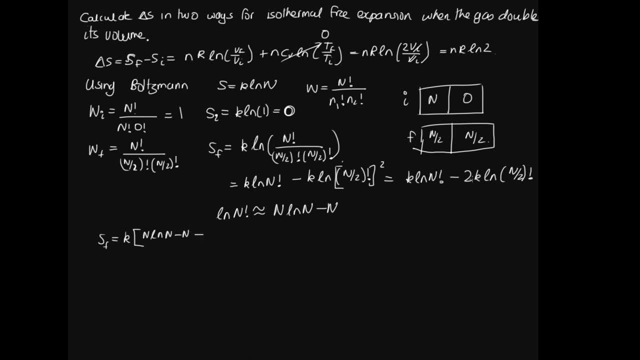 minus. okay, we've pulled the k out the front, but we've still got the two. so this is then two times. now we've got n onto here, so this is n onto log, n onto minus, but it's minus minus, so it's plus two. that's that two, and then this is n onto okay. so now we want to simplify a bit here. we've got a. 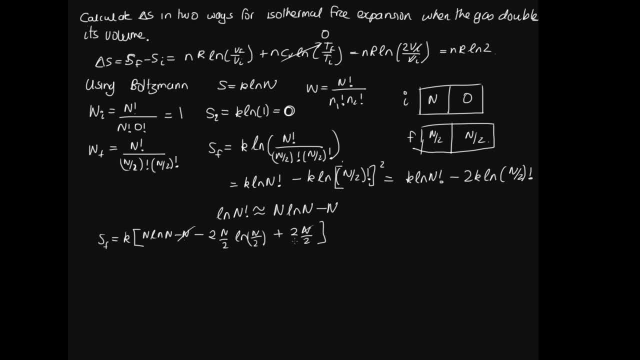 minus n, and this thing here is a plus n, so that cancels that, and so we have k n log n minus. this is these twos cancel. so this is equal to n log n onto. okay, so let's pull n out the front. so we've got k n, and then we've got log n minus log. 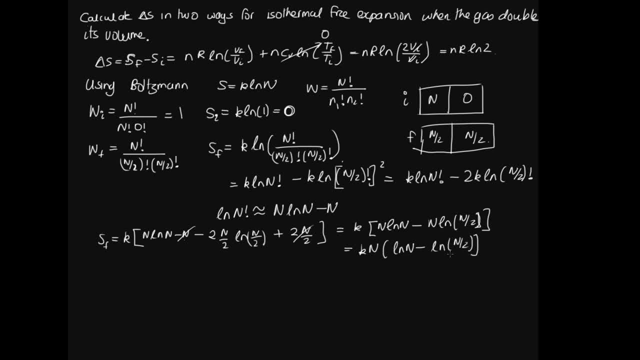